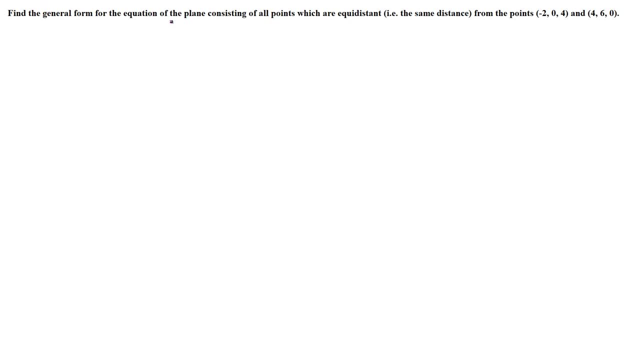 Find the general form for the equation of the plane consisting of all points which are equidistant from the points, these two points. So general form for the equation of the plane is just ax, plus by plus cg equals some constant d. where a, b, c is, the is a normal vector. okay, so to find the equation, to find the equation. 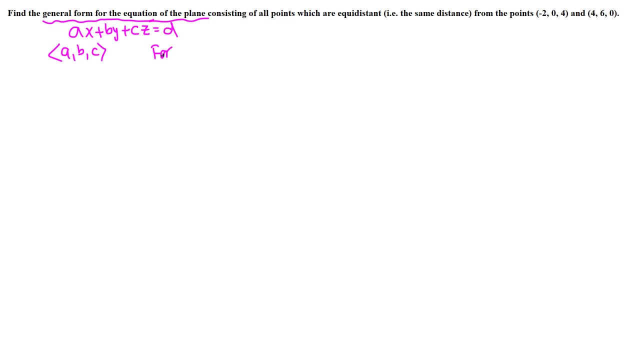 we need two things. okay, for we need need two things: a point on the plane, okay, this x naught, say x naught, y naught, g naught, and normal vector a, b, c and, if we read this question carefully, our plane, I don't know where. 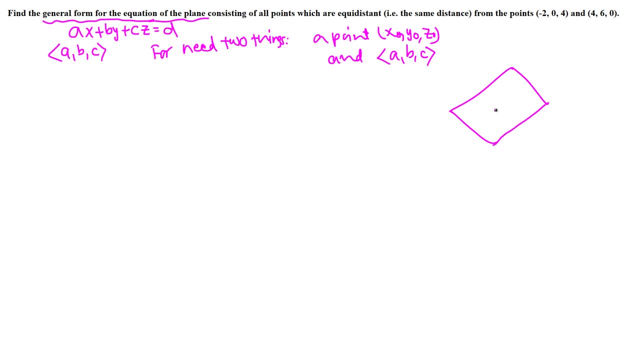 but somewhere like this: all the points, okay, on this plane are equal, equidistant from these two points. obviously one point should be here like negative, two zero, four on the one side and the distance here, and another point on the other side, four, six, zero, okay, so that these two 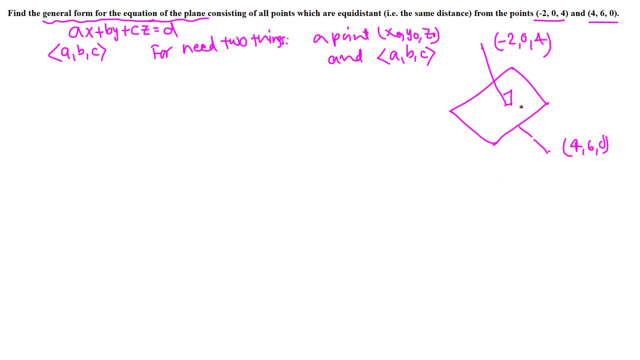 distances are the same. that means if we find find the midpoint of this line segment, if we find the midpoint of this line segment, that midpoint should be on the plane. so our point, that's what we are looking for, this point is just the midpoint. So let's find that here: midpoint of or just midpoint. we know the context of the line. 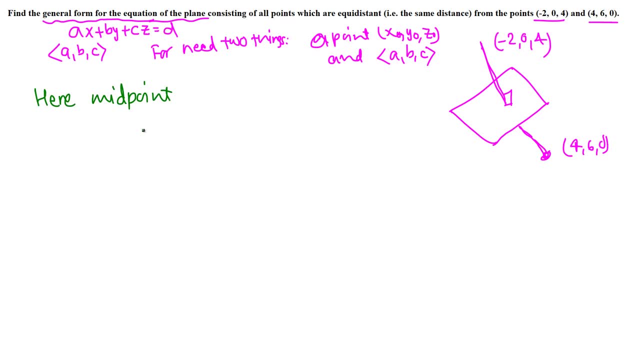 segment. joining these two points is equal to. we just add the corresponding components and divide by two negative. two plus four over two, that's x, zero plus six over two. four plus zero over two, That is four. one, three, two. so this is a point on the plane, so this part is done. 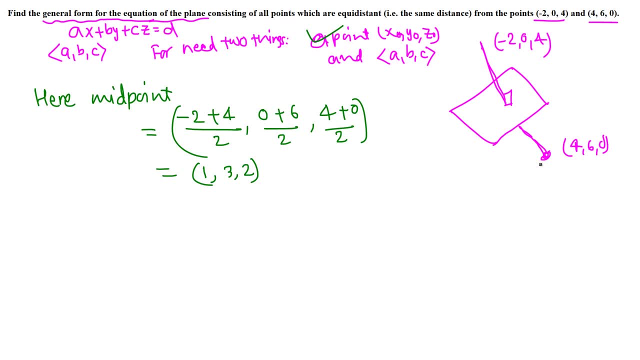 now we need a normal vector abc and let's say this point is p. okay, if we say this point, p and q find the vector pq. since these are distances, that means perpendicular distances, this vector will be normal to this plane. okay, so vector PQ, we are assuming the first. 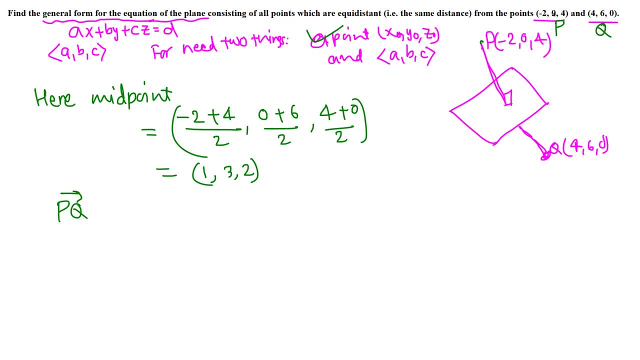 point is P doesn't matter which one is which- okay, PQ or PQ, then PQ is just now 4 minus negative 2, 6, 6 minus 0, 6, 0-4, negative 4. so this is normal vector. that means a, b, c for our equation- and this is a point on the plane- x, not y, not g, not. 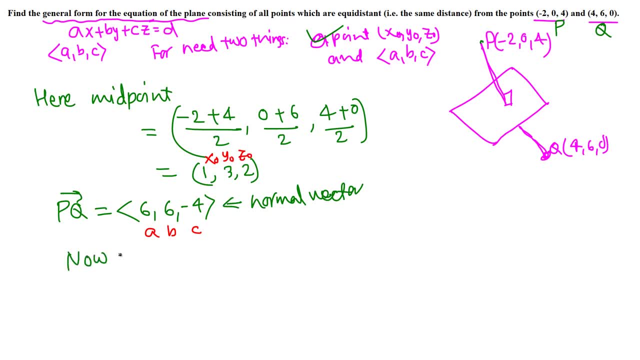 now, and equation of the plane in the scalar form or in standard form, is we first write in the standard, a standard form, then later convert into the general form. so ax minus x, naught plus b, y minus y, naught plus c, g minus g naught equals 0. 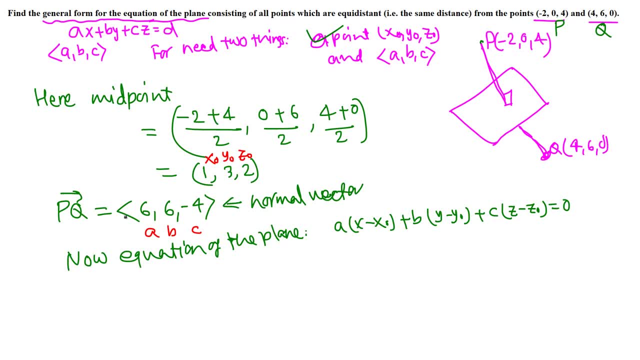 a, b, c are the components of the normal vector 6, 6 negative 4. in fact, we can make it a smaller. we can divide through by 2 and get 3, 3 negative 2. that is also a normal vector. okay, we can just divide by 2 and we get that same as 3, 3. 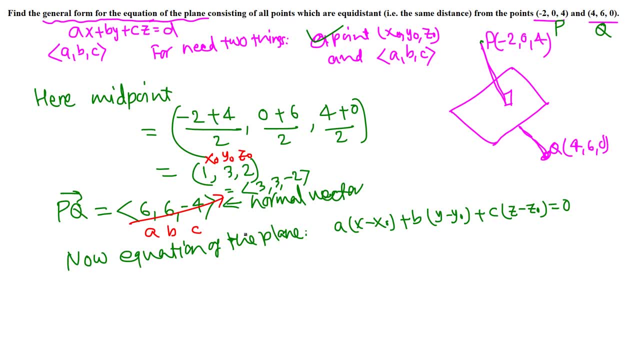 negative 2. okay, Because we have a normal vector and we can divide by 2 and we get that same as 3, 3 negative 2: okay, because we can always divide or multiply by a negative number and we still get a normal vector. so 3, 3 negative 2. 3 ax minus x. naught is 1 plus b is 3 y minus.